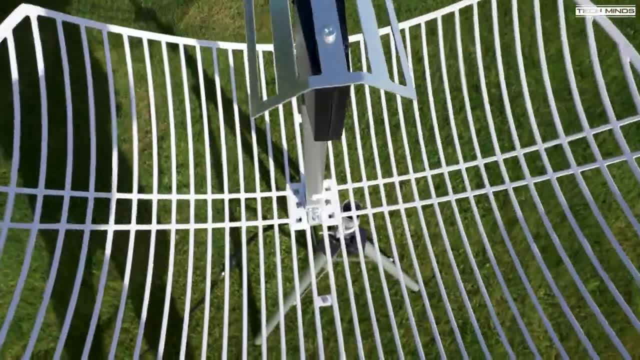 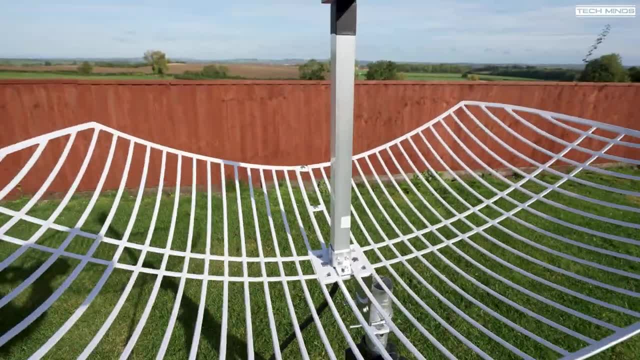 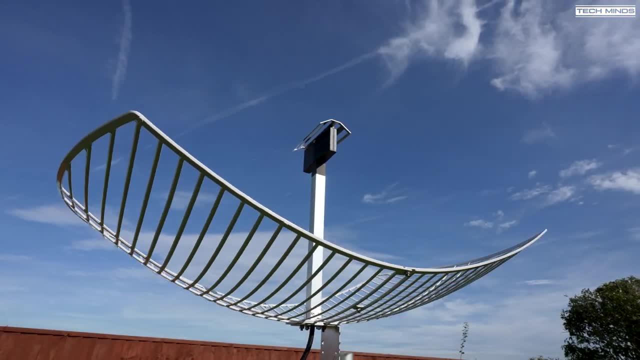 is electromagnetic radiation at a frequency of 1.42 gigahertz which can be detected from earth. Now this explains why I have this antenna pointing directly up into the sky. Now I don't have a calculator to change its elevation, so it's just fixed pointing up for now. Now, using this dish. 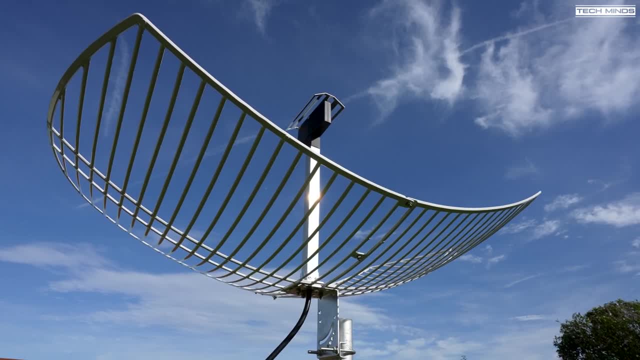 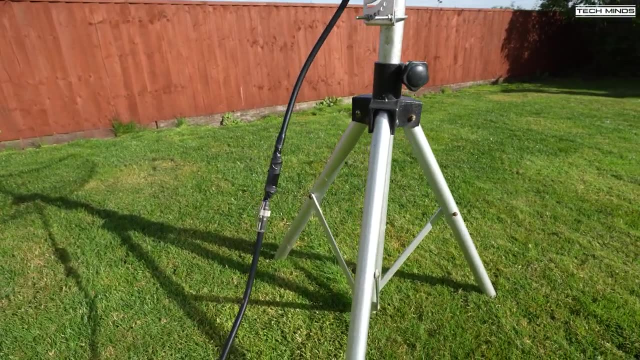 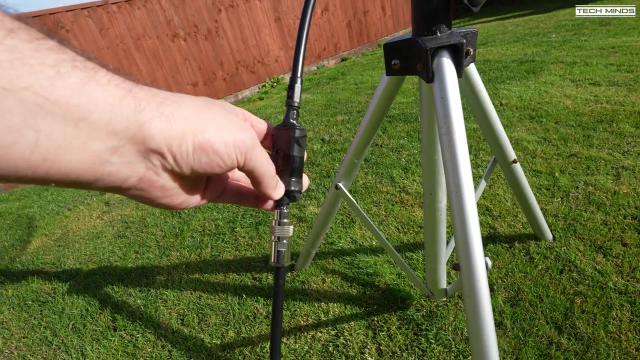 size means the signals from the hydrogen line are fairly weak. but to help improve our chances of seeing these signals we need to use a sawbird filter and a low noise amplifier designed for use at 1.42 gigahertz. Luckily, Neueleck manufacture and sell a device specifically for this purpose. 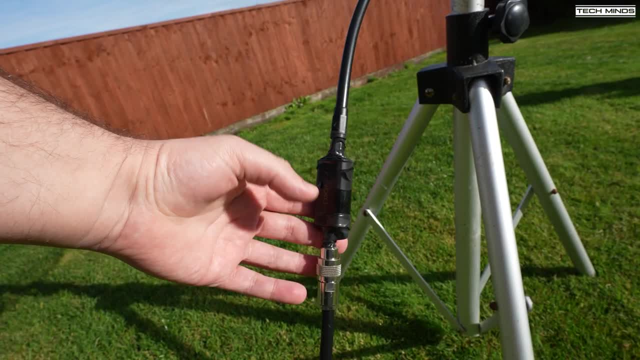 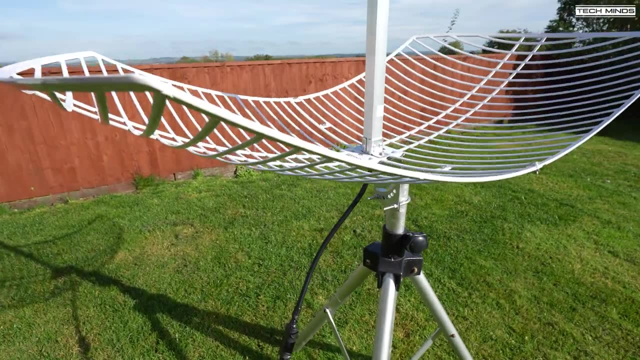 and I have this attached at the antenna end. Now this is a satellite mesh antenna from Neueleck. Now this is called a sawbird plus h1 and it's available for purchase on many places like Amazon. I'll leave a link below to make it easier for you to find it if you want to try it. 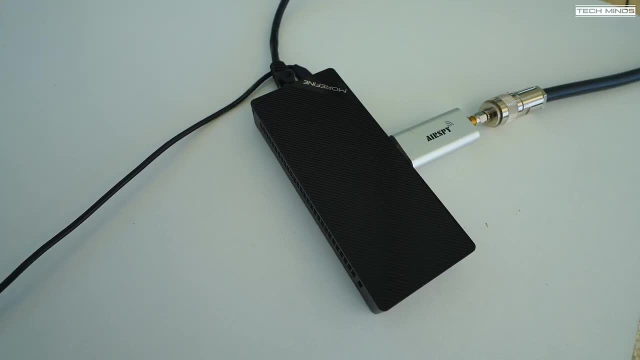 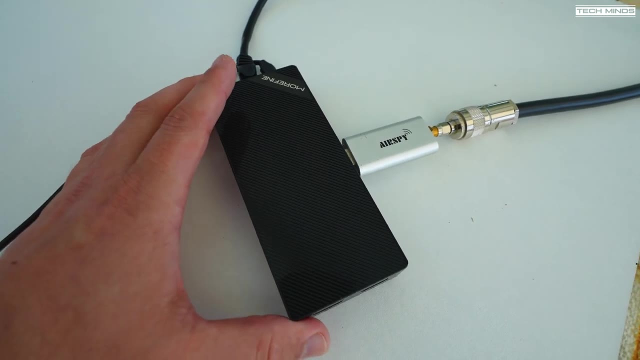 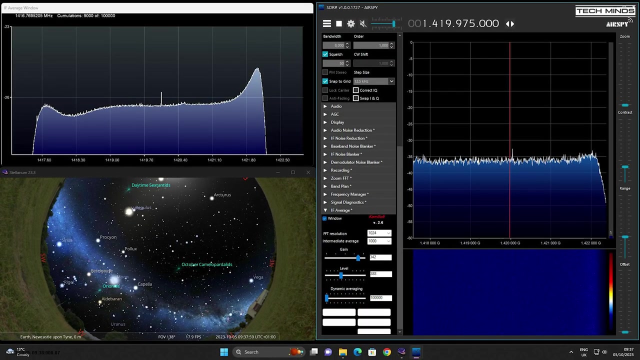 Using a run of formula zero, low loss coax goes off to an SDR receiver which is plugged into a little mini pc which is running windows 11.. Now on this pc we're using an older version of SDR sharp. for this is because we need to use a plug-in called IF average. Now this plug-in didn't seem. 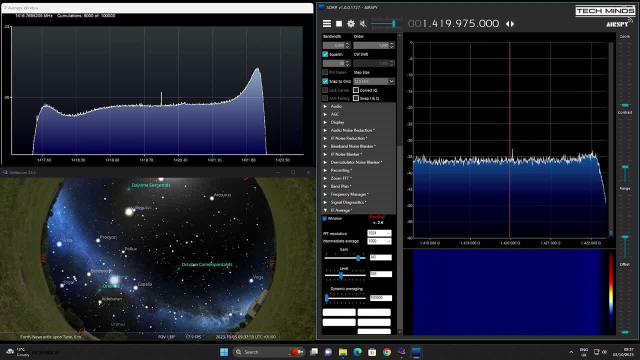 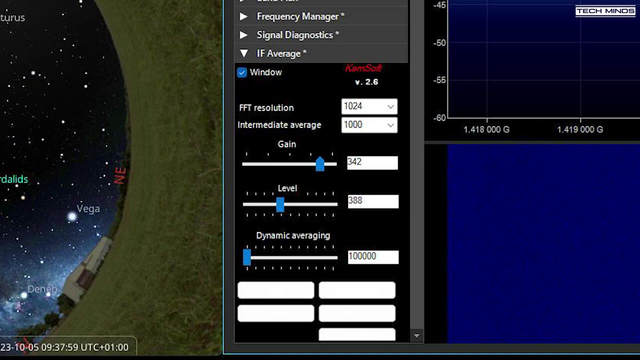 to work too well for me on this pc with the latest version of SDR sharp, but maybe you'll have better luck than me. but if not, you can use the same version as I did and use 0.1727.. Now I set the FFT resolution on the plug-in to 1024 and the intermediate average to 1000.. Now gain is set to. around 350 and level is set to 100.. Now I'm going to set the FFT resolution to 100.. Now I'm going to set the FFT resolution to 100.. Now I'm going to set the FFT resolution to 100.. Now I'm going to set. 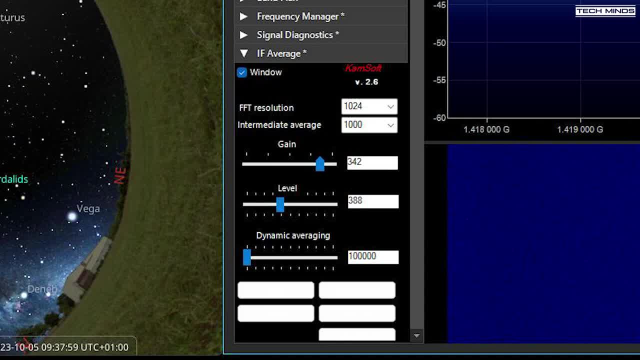 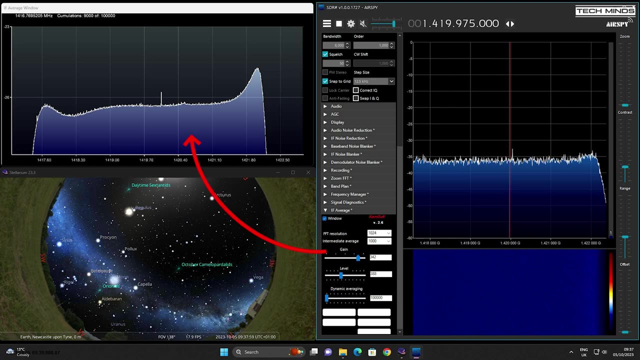 around 400.. Now there is a procedure in which you perform a background noise scan without the antenna connected before you start using this software. Now the window on the top left is the output from the IF average plug-in, and it's here where we will hopefully see the 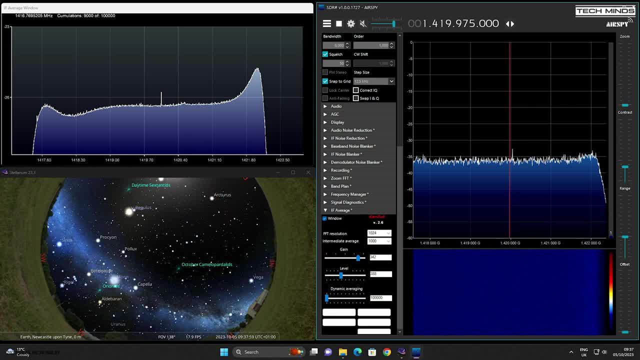 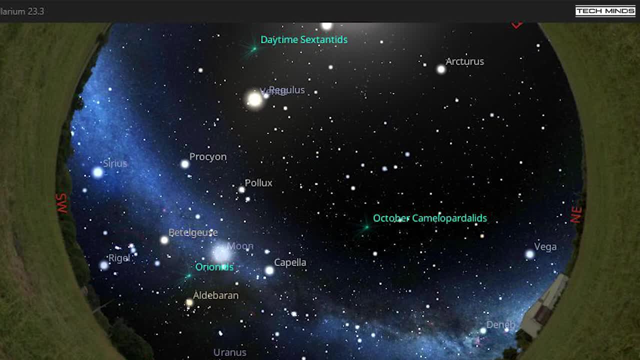 hydrogen line appear So that we can visualize the orientation of the Milky Way. I've installed an application called Stellarium. Now, luckily this is a free application- Pointing the virtual camera within Stellarium towards the sky. you should be able to virtually see what's above you, assuming you have your location correctly set within the software settings. 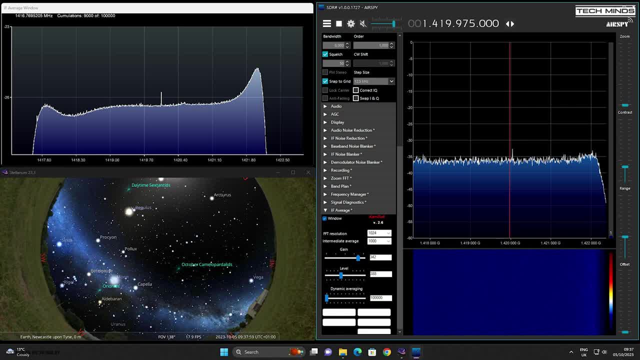 Now, as this is an extremely slow process, I left this running for a good 24 hours Now. I used a free application called chronolapse, which took a screenshot of the computer's desktop every 60 seconds. After 24 hours, I booked a free application called ChronoLapse, which took a screenshot of the 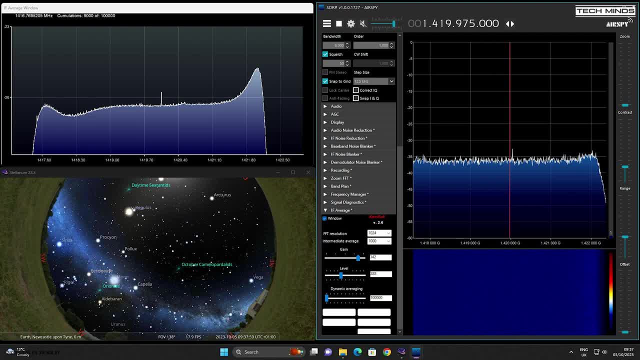 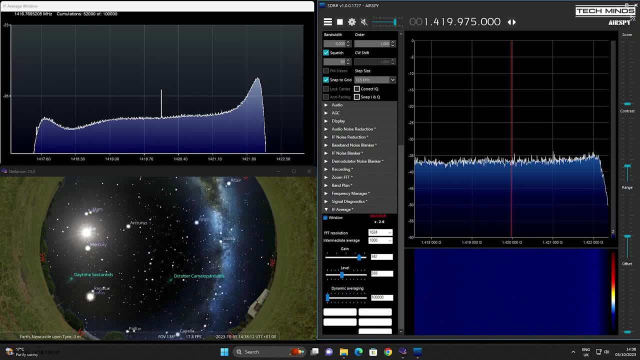 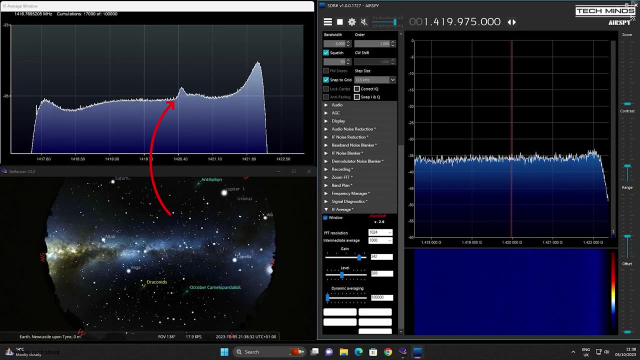 computer's desktop every 60 seconds. Now I'm going to put all of those screenshots into a time-lapse video and here are the results. Now you can clearly see the peak appearing here, which is the detection of the hydrogen line. Now watch how it shifts frequency. This is most likely due to Doppler. 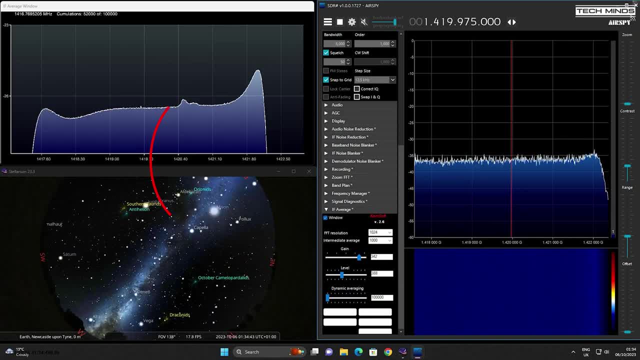 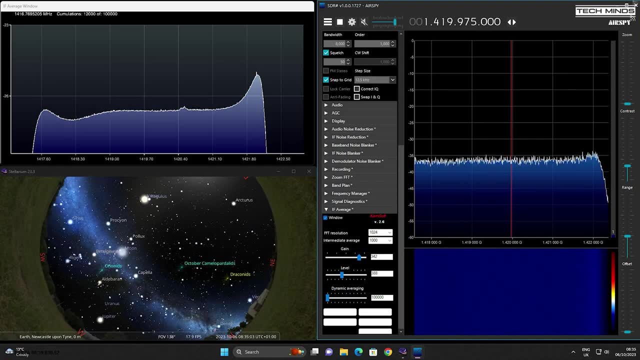 effect as the earth is spinning. Other peaks and spikes shown on the IF average window are most likely local interference. But watching this back after many hours, I'm sure you'll be able to see the results of the experiment Now. as this is an extremely slow process, I left this running for a good 24 hours. 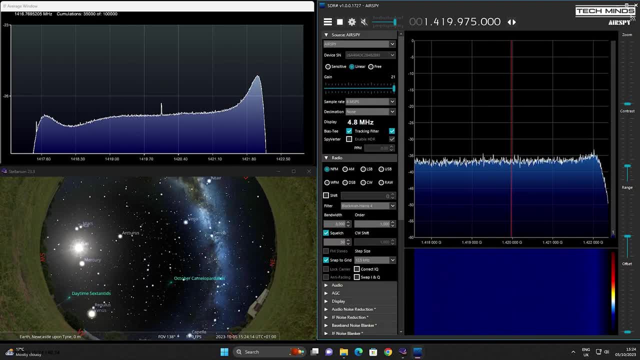 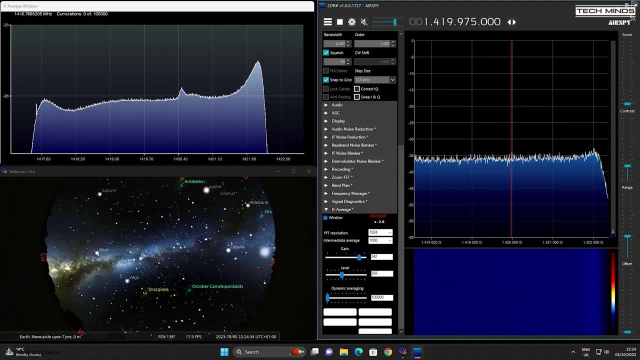 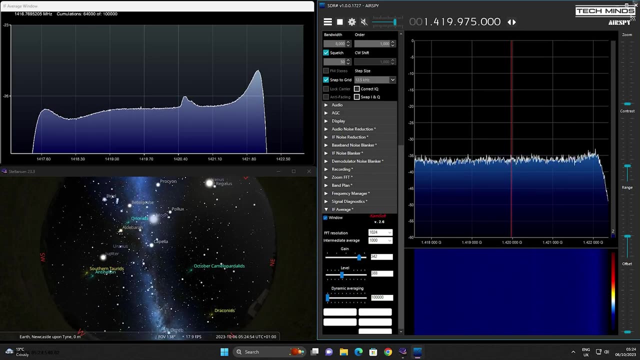 Definitely puts a smile on my face and a sense of achievement. Now, while this may not be the most exciting thing to look at and observe, it's still a fascinating project that you can do at home with minimal equipment. Now, when you start reading through the science of why this happens, it's 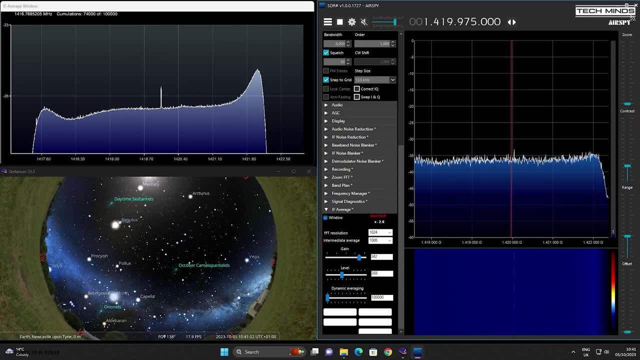 actually quite mind-blowing, even how it was discovered way back in the 1930s, So this may be the start of a new era of video games. Now I'm going to show you how I did it, So let's go ahead and take a look at some of the projects that I've discovered in my radio astronomy journey. 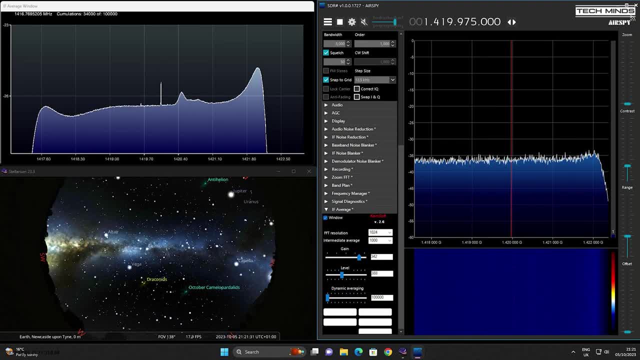 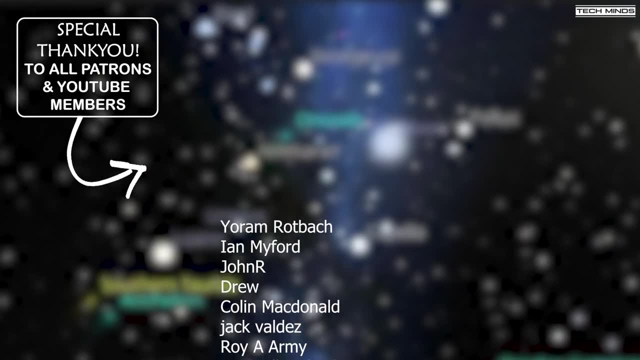 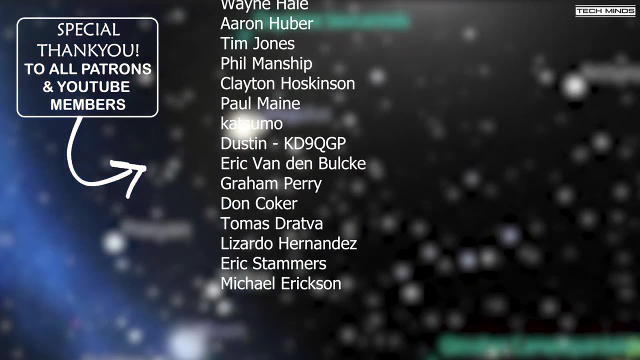 If you like this kind of content, then please feel free to subscribe. If you already experiment with radio astronomy, let us know down in the comments below what you've discovered and what other projects you think I might be interested in and might be worth showing to others. Until the next video, take care and thanks for watching. Bye.